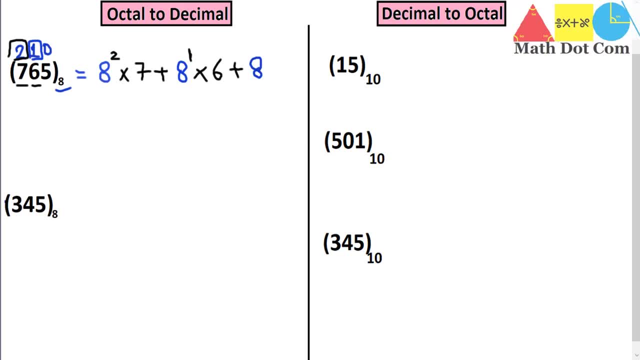 This is the basically base. this base and 8, and now the power is 0.. So 8 to the power 0 multiplied by this number 5.. So what we will get is 448 plus 8.. Plus 48 plus 5, as 8 raised to the power 0 is equal to 1.. 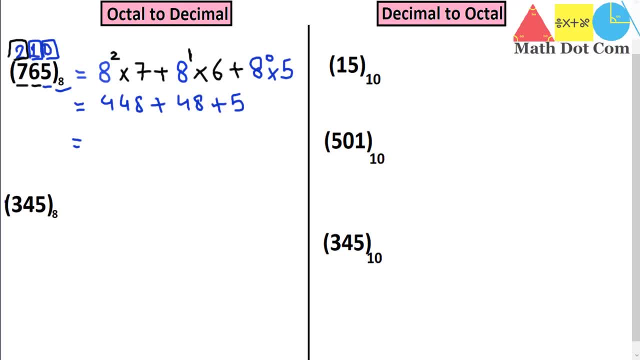 And finally what we will get. the number in decimal form is 501.. This is the decimal equivalent of the number 765.. Similarly, we have to apply the same approach in the next number, that is, 345.. Where again, they are at location 0, 1 and 2, as the base is 8.. 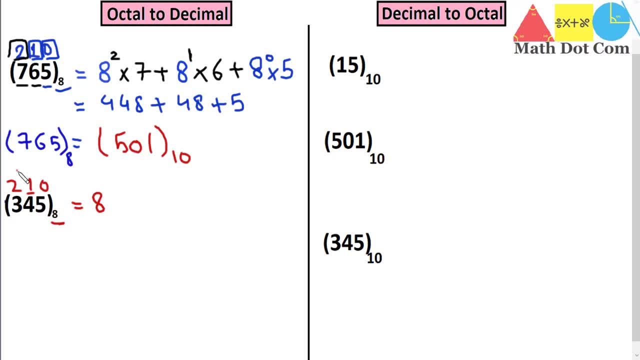 So we have to write the 8.. The power of 8 will be this location: 8 square, multiplied by the number at that location, that is, 3 plus again 8.. The power will be the location 1 multiplied by the number at that location, that is, 4 plus again 8, raised to the power 0.. 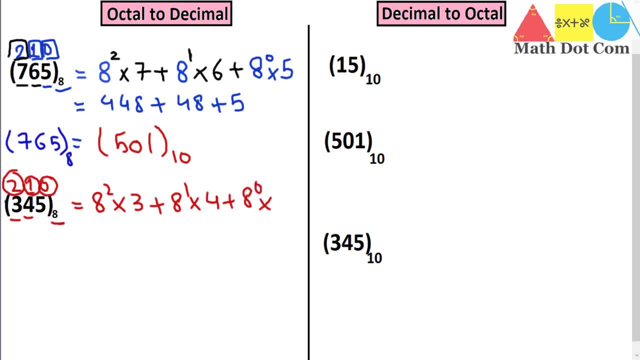 That is the value of that location, 0, multiplied by the number at that location, that is 5.. So what we will get is 192 plus 32 plus 5.. The answer will be 229 with the base 10.. So we have converted the octal number 345, the base 8, into a decimal number that is equal to 229.. 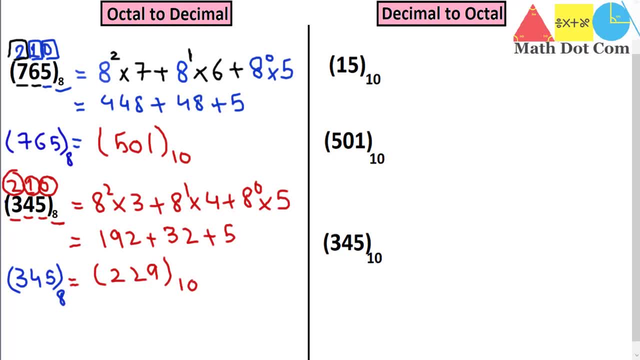 So this is the method of conversion. Now we will convert a decimal number. We will see how we can convert a decimal to the octal, that is, a base 10 to the base 8.. So its method is very simple. What we have to do, 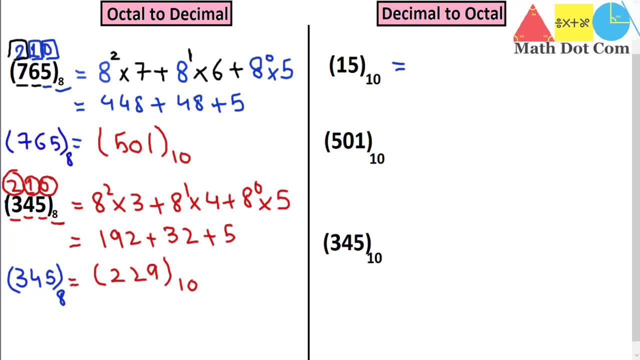 We have to do a repeated division of the number by 8. Because we are going to convert it into octal number. So I will write 15 and do a repeated division, as 8 ones are 8 and the remainder is 7.. 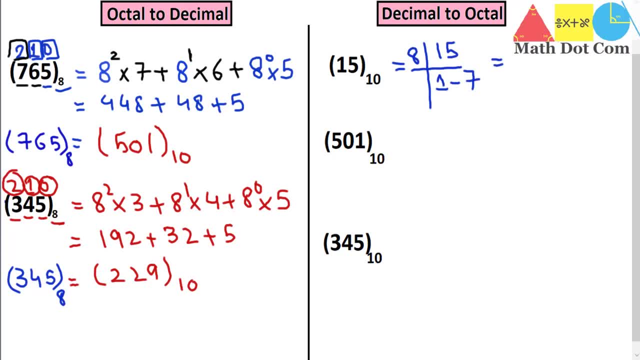 So what we will get is we have to, as we have to write in this manner. So the octal equivalent will be 17 with the base 8.. Similarly, we have another number, that is 501.. We have to do the repeated division of 501 by the 8, as we have done in the example number 1.. 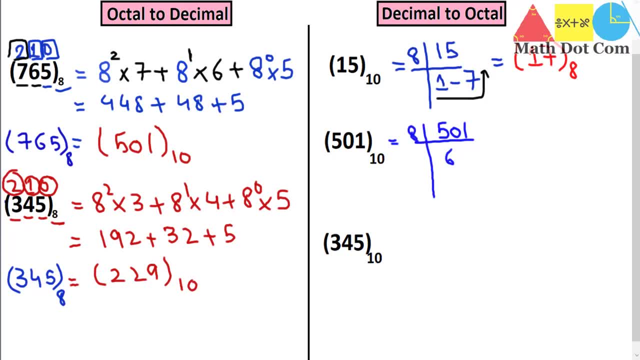 So 8, 6s are 48, 21, then 8: 2s are 16 and the remainder will be 5.. Again, we will do the division: 8, 7s are 56 and the remainder will be 6.. Now we can't divide it further. 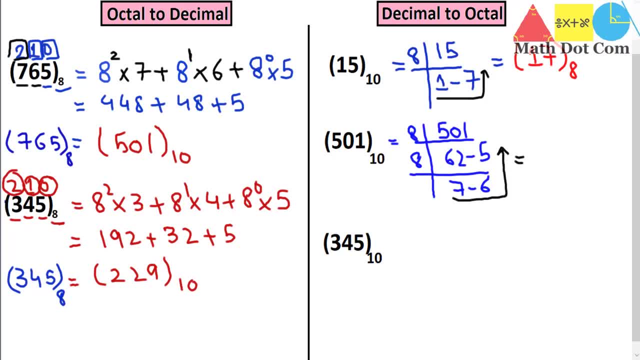 So we will write it in this manner, and what we will get is 7, 6, 5.. This is the octal equivalent of the given decimal number. Now we move towards the last example: 3, 4, 5.. What we have to do? 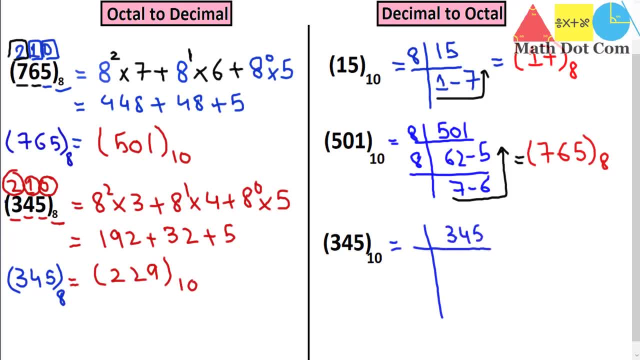 We have to again do the repeated division with the remainders, As 8: 4s are 32, 25, 8 3s are 24, remainder is 1.. Then again we will do the division: 8: 5s are 40 and the remainder is 3.. 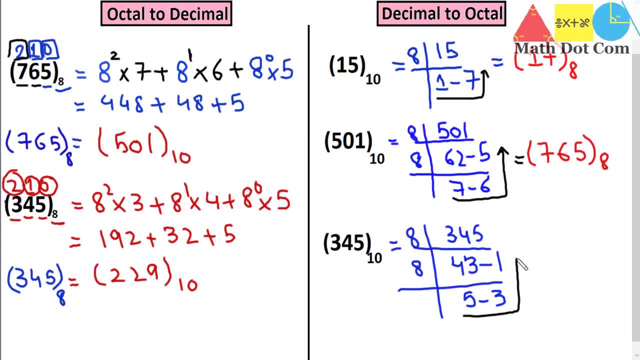 So we have to stop the division here, as we can't divide it further. So what we will get is the decimal equivalent, that is equals to 5, 31.. So this is how you can convert octal to decimal and decimal to octal. That's all from today's lecture. Thank you. 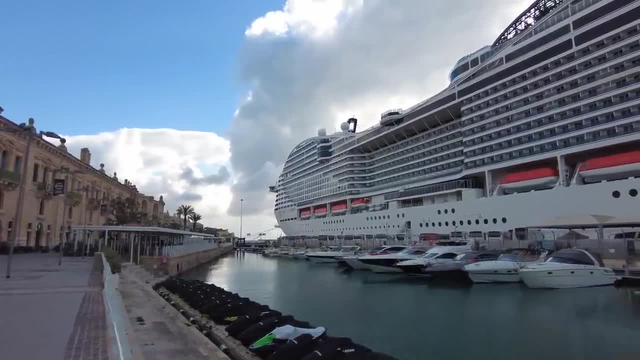 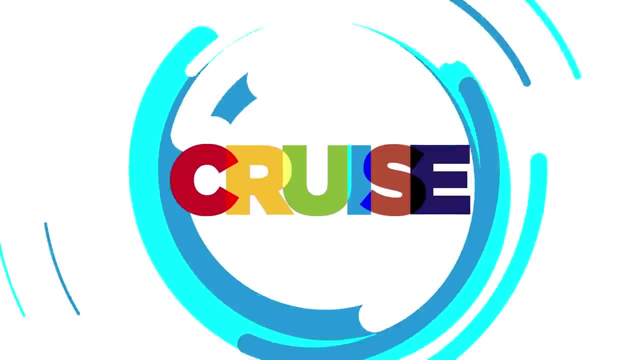 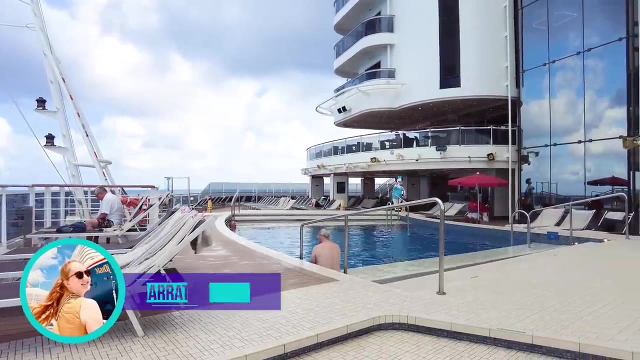 Hey everyone, welcome to Cruise Blog. This is Angie, and today I'm going to be talking about why MSC Cruises are so cheap. Let's get started. Do you want a cheap cruise? Well, MSC Cruises might be what you're looking for. 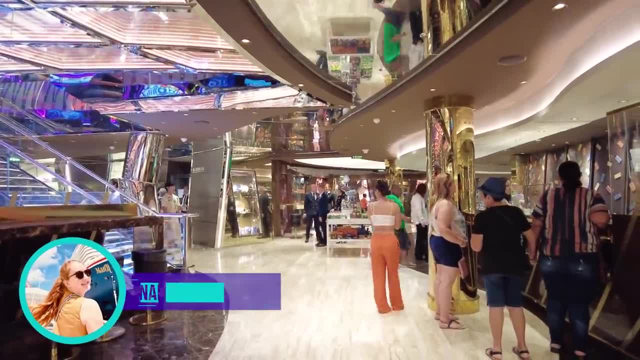 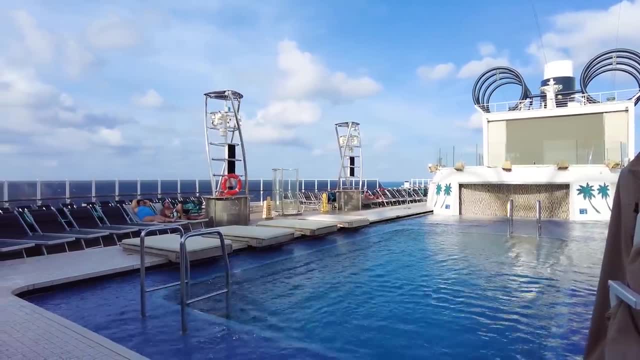 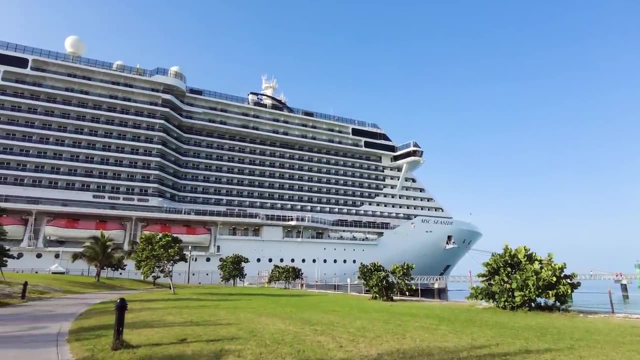 They have some of the lowest cruise fares around, even beating Carnival Cruise Line, who's known for offering a great value. MSC Cruises has become increasingly popular, especially in North America. Not only do they have some of the best budget-friendly cruise prices, but they also often include add-ons like basic Wi-Fi and drink packages as part of their promotions luring cruisers from other cruise lines. 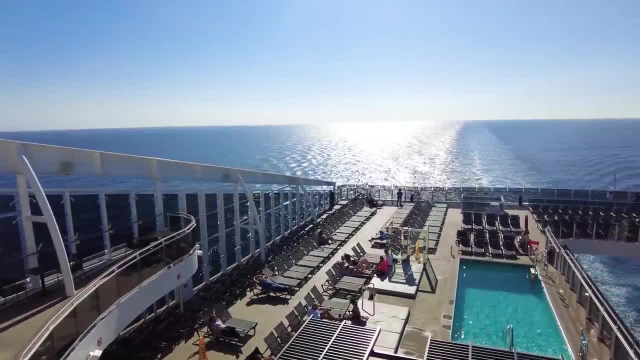 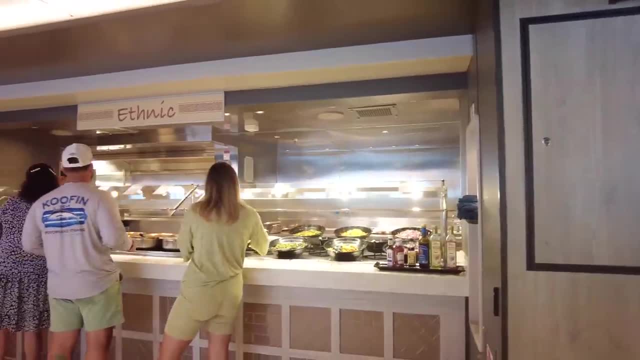 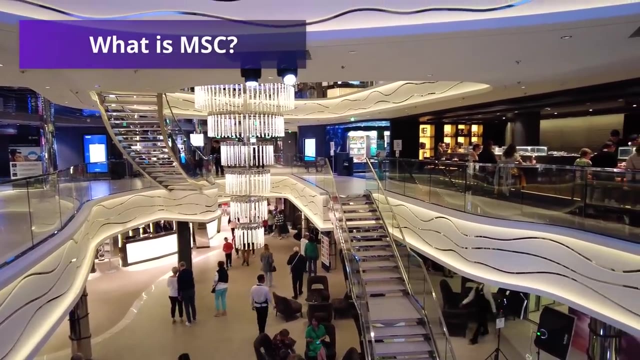 But why are MSC Cruises so cheap? What's the catch? Let's take a look at how MSC Cruises can possibly deliver these discounted fares and what cruisers need to know when sailing with this European cruise line. First, let's discuss MSC Cruises: Who are they and who owns them? In fact, they are the largest privately-owned cruise line in the world. They are part of the Larger Mediterranean Shipping Group. They have over 180,000 staff worldwide and 760 ships- a maritime giant, to say the least. MSC Cruises currently sails to over 100 countries with 22 cruise ships and another 5 due by 2027..